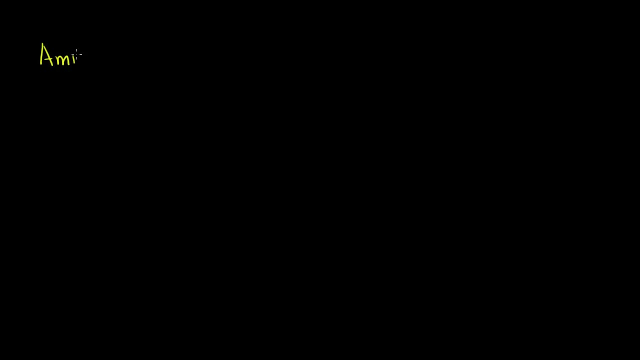 In this video we're going to talk a little bit about amines, And these are just organic compounds where you have a nitrogen bonded to groups that contain carbon. So if I were to just draw some amines right here, you could. 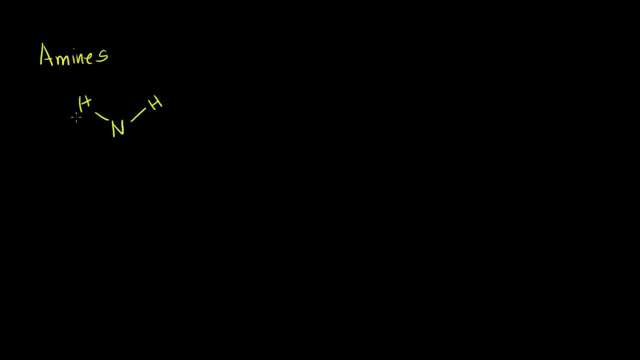 have something like this, where you have a nitrogen bonded to two hydrogens and then maybe some type of carbon chain. maybe it's just one carbon right here, So maybe you have a carbon which is also bonded to three hydrogens, like this: 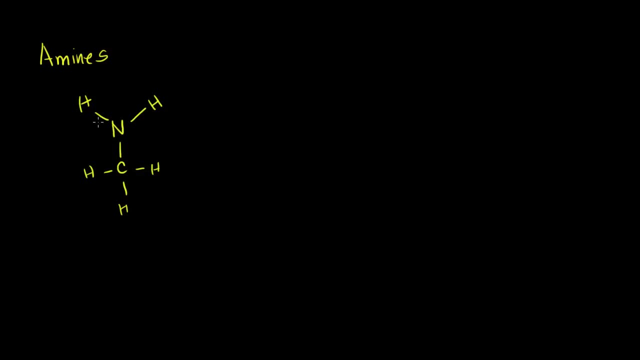 In this case you would have a primary amine If you have the nitrogen bonded to two carbons. so if you have something like this, a nitrogen bonded to two carbons, so it has one carbon chain right there. And I'm just drawing methyl groups here, because the chain 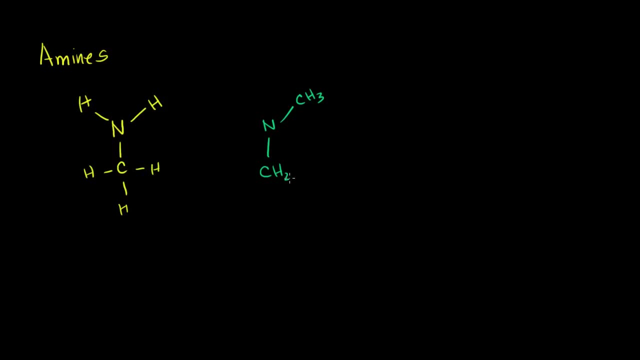 could keep on going. Maybe you have two like that and then you have a hydrogen right there. This would be a secondary amine And then, finally, you could imagine if you had it bonded to three, it would be a two Tertiary amine. 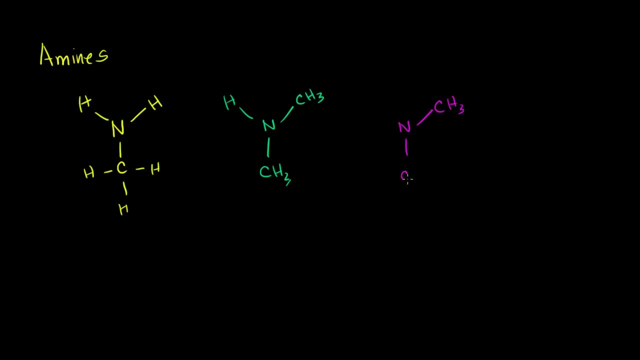 And this is just to get you introduced to the terminology, Just like that. Now, like all of the other new groups or new types of compounds that we've explored, what I want to do is just introduce you to the naming of it, Because one that lets you recognize them when you hear. 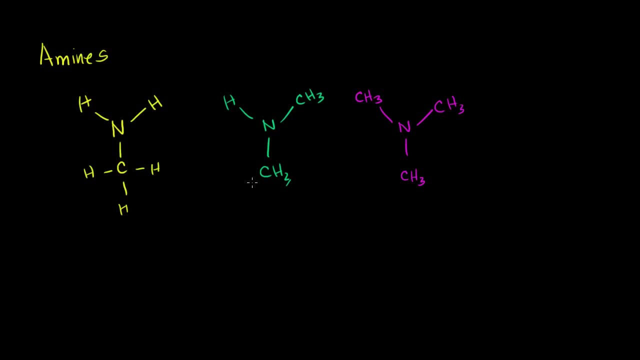 their names, but it also, I think, on some level familiarizes you with their structure. So let's do a couple of naming examples. I drew these ahead of time And in general. just to remember, amines are a pretty 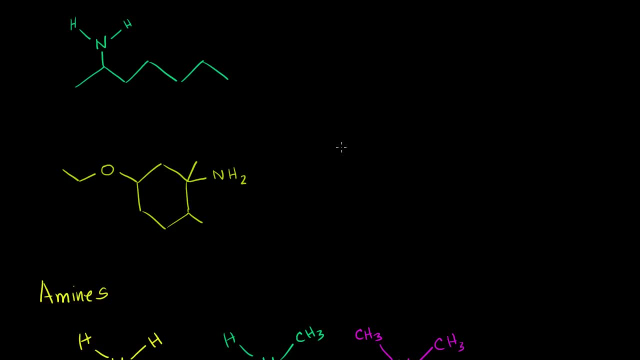 high priority group. Out of all of the things that we've learned so far, the only thing that is a higher priority is actually the alcohols, or actually the thiols, which I don't even remember if I did a video on it. 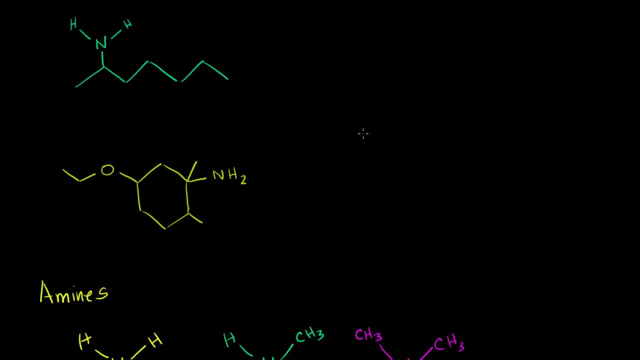 But thiols are just like alcohols, but instead of an oxygen you have a sulfur, So this comes right after those. So let's think about this one right here. So we always want to look for our longest carbon chain and 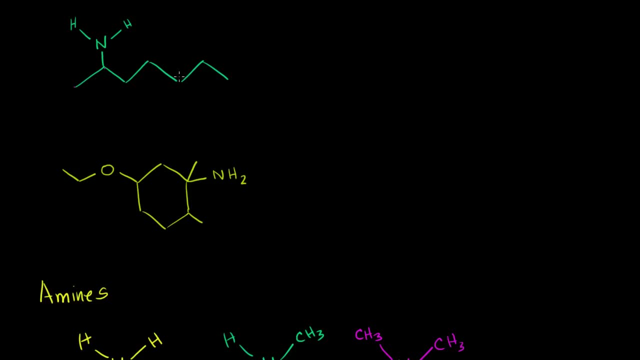 our longest carbon chain. Our longest carbon chain is right here: One, two, three, four, five, six, seven carbons. You want to start numbering it closer to the functional group: One, two, three, four, five, six and seven. 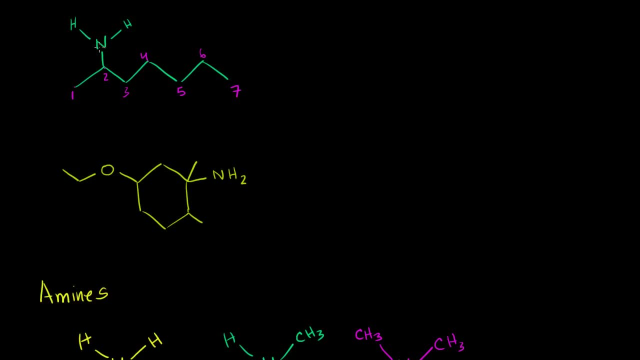 And then the functional group is on the two carbon right there. So first of all seven carbons. we would use the prefix hept, So it would be heptan. Let me write that down. So it would be heptan. 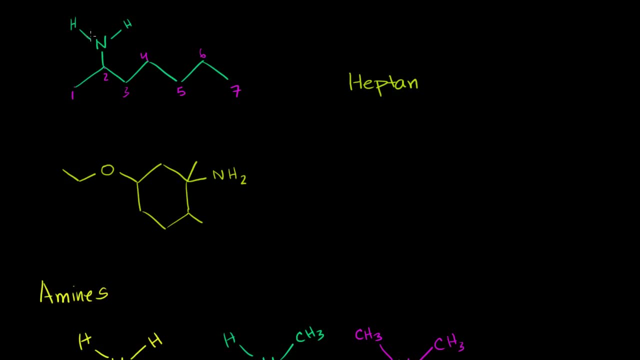 And since our functional group is an amine in this situation, it has a higher priority than the fact that this is an alkane, so this will actually define the suffix. So we would then say: well then, on the two carbon right. 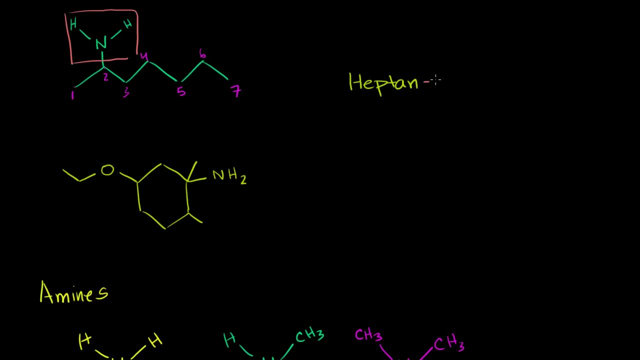 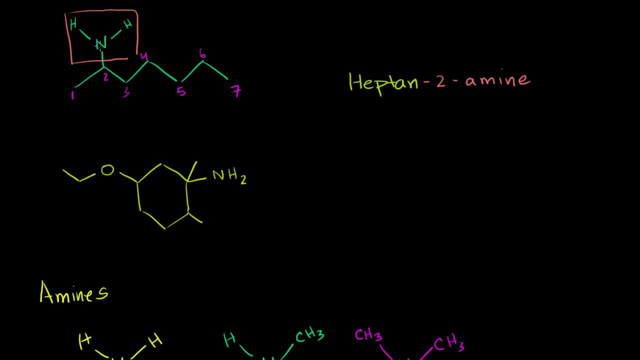 And we're done. We know that we have an amine group on the two carbon. Now let's do this one. This one's a little bit more hairy. So first of all, we always want to figure out the longest carbon chain. 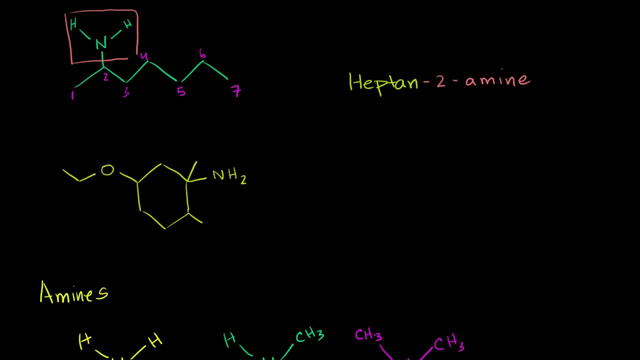 And it looks like the ring is going to be the longest carbon chain. We have one, two, three, four, five, six carbons, So this thing right here is the longest chain. We only have one, two carbons right there, one carbon one. 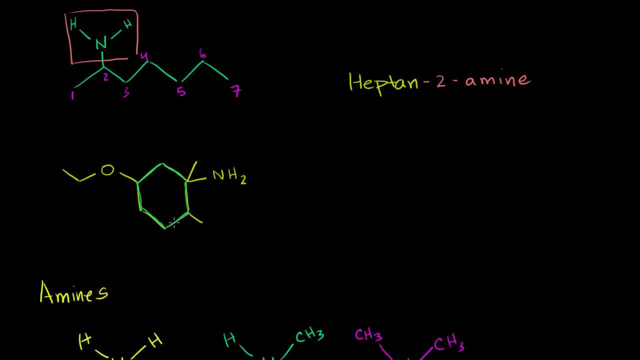 carbon right over there. So our root, Our root is going to be cyclohexane. So our root is going to be cyclohexane. I want to make sure I have enough space: Cyclohexane, And then, once again, it's an amine. 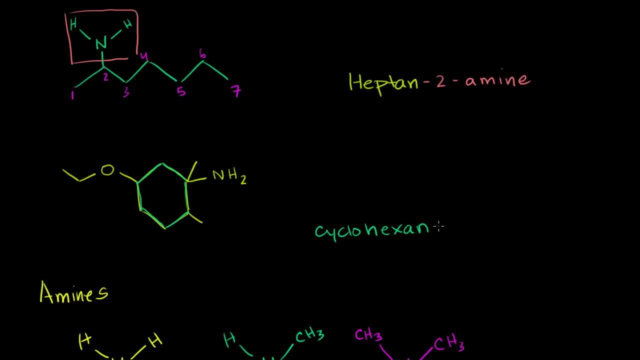 So this is going to take higher priority. So we're not just going to put an e at the end and call this cyclohexane. This takes higher priority, So it'll actually define the suffix. And another thing to think about is: you could. 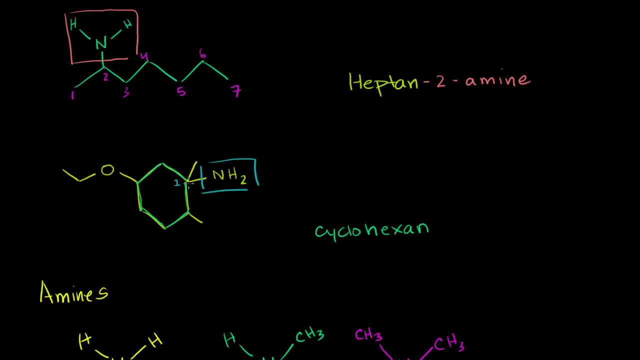 say: OK, this is going to be the one carbon, And so you could call this cyclohexane one amine. But in general, if this is defining it, you always assume that you're going to start numbering right there, at number one. 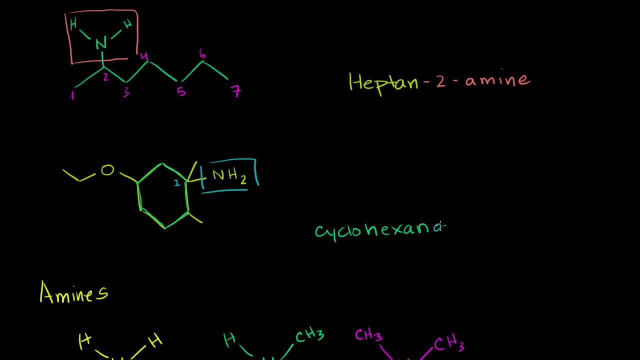 So you could just call this cyclohexane amine. If it's written like this, you assume that the one carbon is where the amine group is attached. Now, what else do we have on this thing? We took care of the amine. 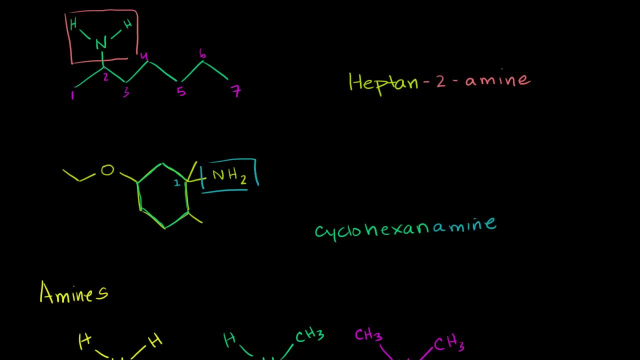 We took care of the cycle. Well, we have this ether right here, And this ether has one, two carbons. If it was just a two carbon chain, it would be ethane, But since we have it's an ether, it's bonded to this. 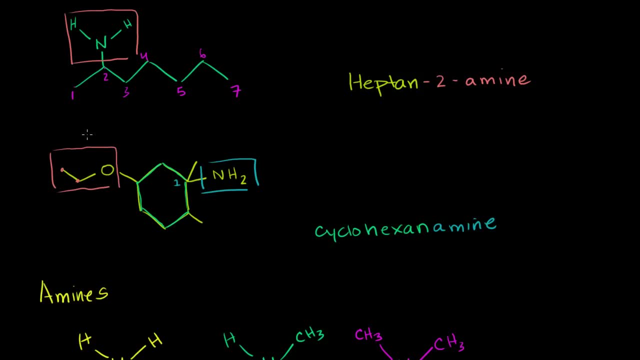 oxygen. we call this ethoxy. So that right, there is ethoxy And we're going to have to think about how we're going to number this, So I'll leave that alone. And what are these over here? Well, this is a methyl group. 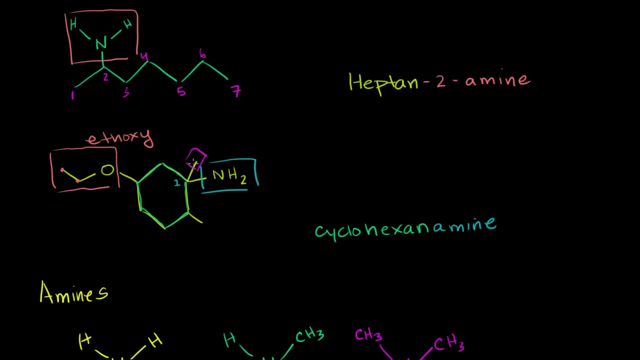 That's a CH3 implicitly. You don't see it drawn. There's a carbon there. If carbon is neutral, it has to have four bonds, And if you only draw one of them, the other three are assumed to be the hydrogen. 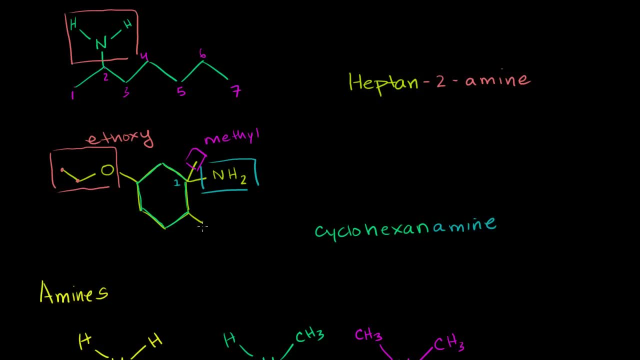 So this is a methyl group. And then this is also a methyl group, So we have dimethyl. So this is also a methyl group right over there. And when we think about numbering, we could number from one, two, three, Or we could start numbering one, two, three. 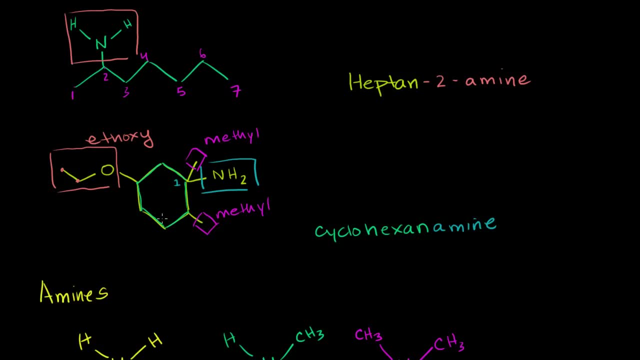 And in general you want to go numbering in the direction where you hit the functional group first, OK, OK. So you want to go one, two, three, four and five. So this right here is 5-ethoxy. 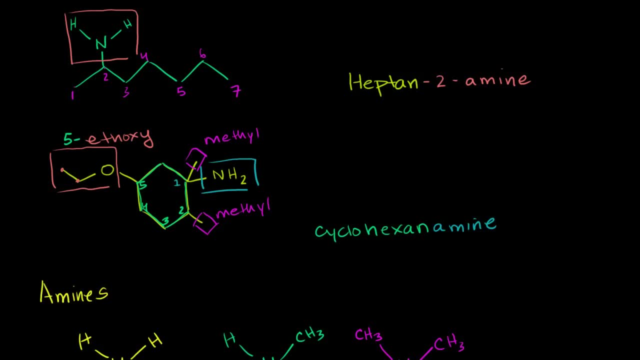 This is 5-ethoxy And then this is 1, 2-dimethyl. These two combined, you would call this 1, 2-dimethyl, And then, when you want to list them in order, the ethoxy. 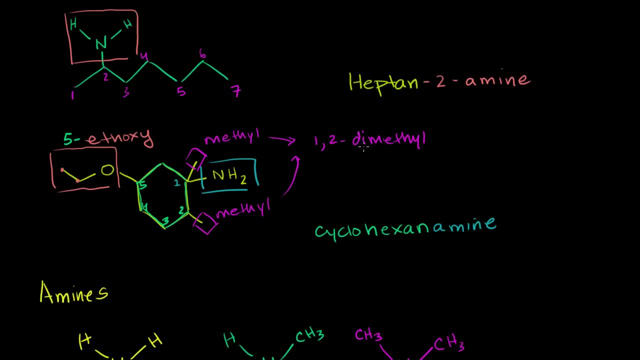 would take precedence in alphabetical, Because the di you shouldn't count in the alphabetical order. This is just saying two methyls, So you really just want to look at the two of whatever you're talking about. M comes after E in alphabetical order. 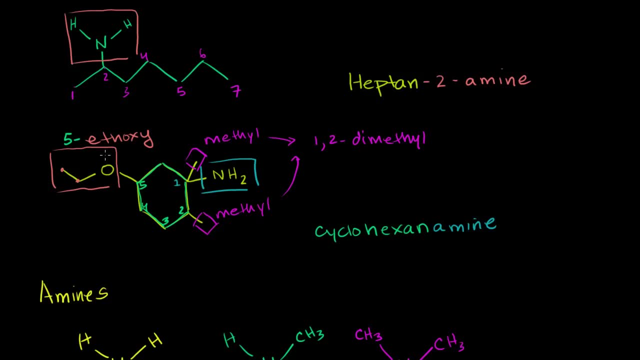 So this is going to be 5-ethoxy. Actually, let me just rewrite the whole thing. So this is going to be 5-ethoxy: 1, 2-dimethyl Dimethylcyclohexanamine.